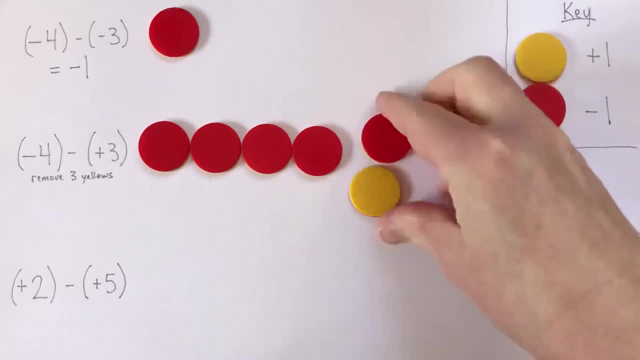 And the way we do that is by using zero pairs. So if I add a zero pair here, this is negative one. two, three negative four, and this is worth zero. So this whole number is still negative four. So we're actually. this is getting us on the right track here. It would be possible now to 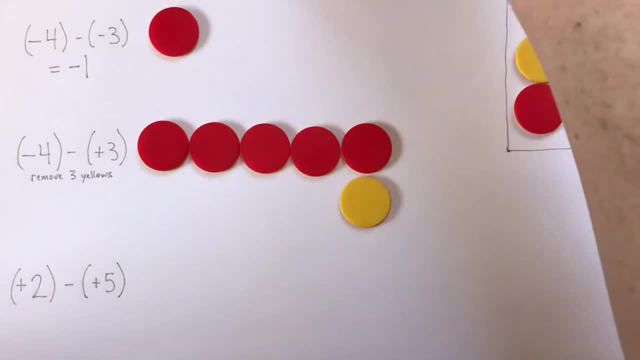 remove one yellow, but we'd like to remove three. So what we'll do is we'll just put on another zero pair. So, as you do this, I suggest telling yourself, even out loud or under your breath: this is still negative four. It's really important to remember that it's still negative four. 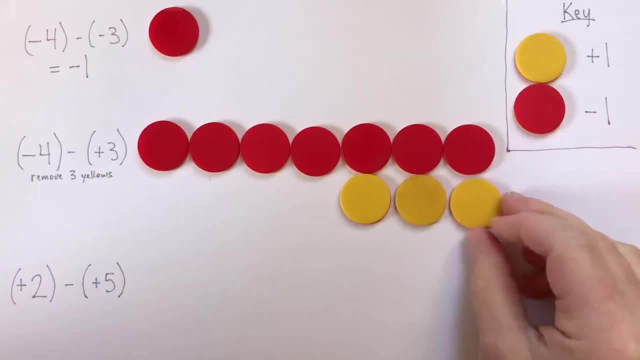 Sometimes people think they go through all this and they think they've already done the subtraction. This here is still negative four, because all of this is worth zero. That's negative. This is negative four And we're doing great now because we have negative four and we have three. 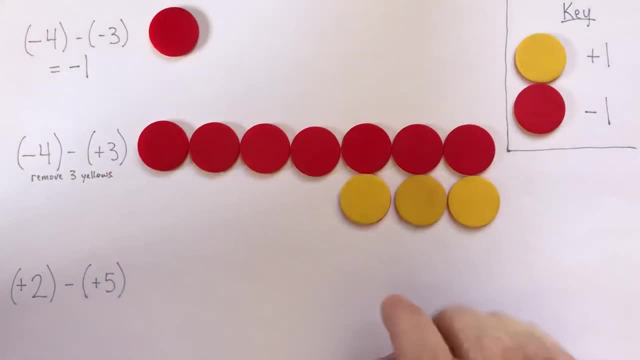 yellows in it, So we can remove our three yellows. So this is negative four. And now I'm going to do the subtraction. I'm going to take away my positive three. So my three yellows I'm going to remove. 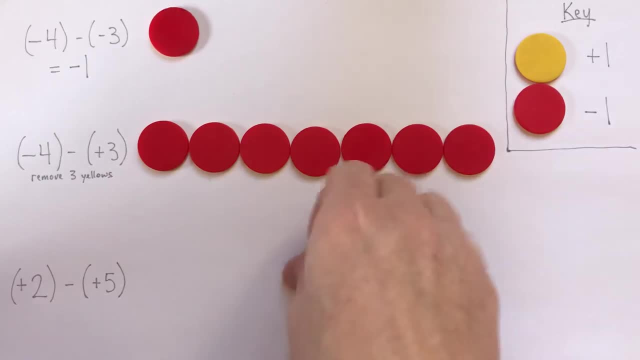 positive three. here And now I have done my subtraction And this is our answer. So our answer is negative one: Two, three, four, five, six, seven, Negative seven. So negative four subtract positive three is negative seven. So even though these two questions looked pretty similar at first glance, they actually were. 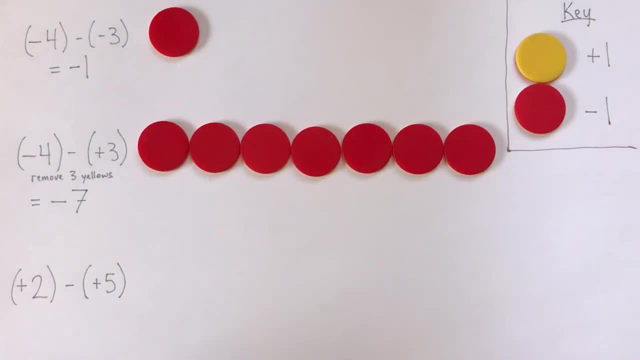 pretty different in how we went about doing them. Okay, let's take a look at another example: Positive two And I'd like to subtract positive five. So here as well, if you look at it, you think, oh, I can't subtract positive five, Not from this. 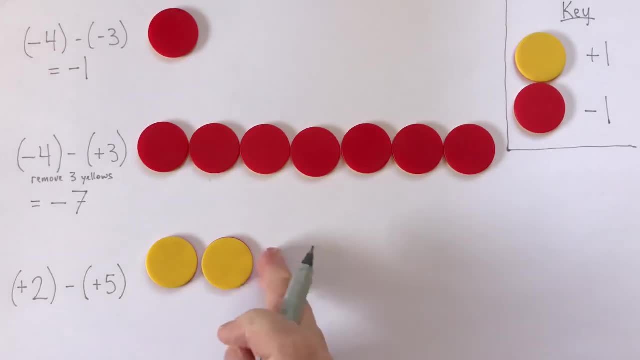 representation anyway, And I just as a suggestion I'd say, you should at least say to yourself, and maybe you should write it down, what you're trying to remove. Here we're trying to remove five yellows, And when we do that that will be the act of subtracting. So, in the meantime, what we're going,